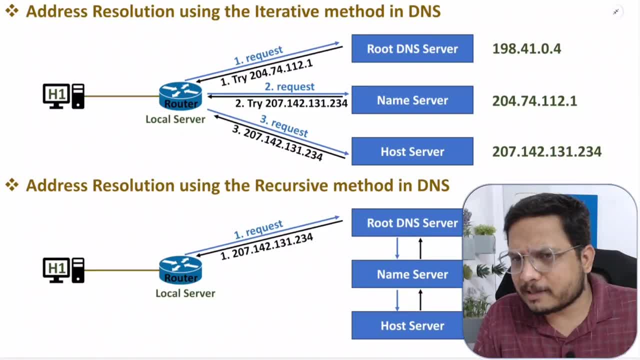 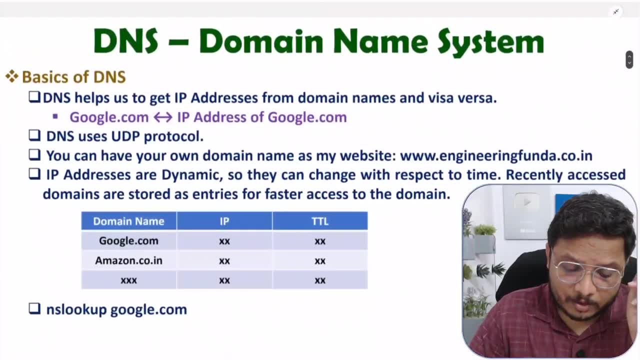 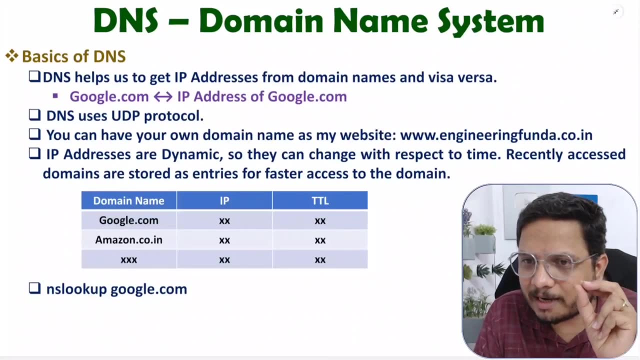 recursive method, that I am going to discuss that in this video along with one practical scenario. so let us try to understand first how basics are there with domain name system. so domain name system that we use it to get IP address from domain names. so first of all you should know what is IP address. there are. 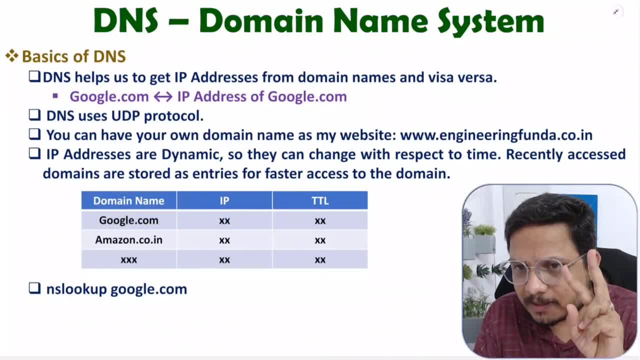 two types of IP address: IPv4 and IPv6 right. and with the use of IP address only one can communicate with another computer. without IP address we cannot communicate on computer network right. so to get IP from domain name we will be using DNS. so what is domain name? domain name means googlecom, that is one. 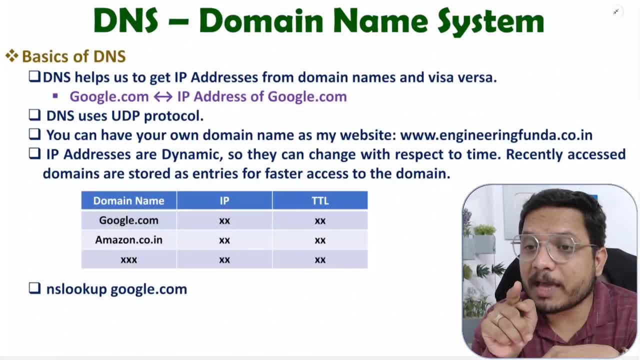 domain name. so to have a communication with Google you should be having IP of Google. to get IP of Google we will be using DNS, right? so when you write wwwgooglecom, you are writing domain name over here on web browser, right, you don't have IP of Google. but to get IP of Google, first DNS frame. that is. 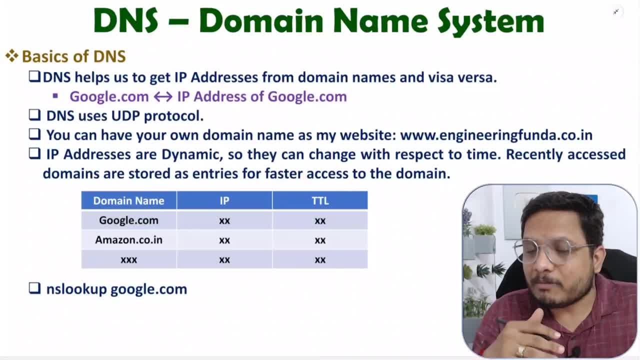 getting forwarded and then DNS reply will come, by which user will get to know IP of Google and now user can communicate with Google. so before communication user should be having IP address to get IP address. DNS is used right. DNS is using UDP protocol. so let me show you that by. 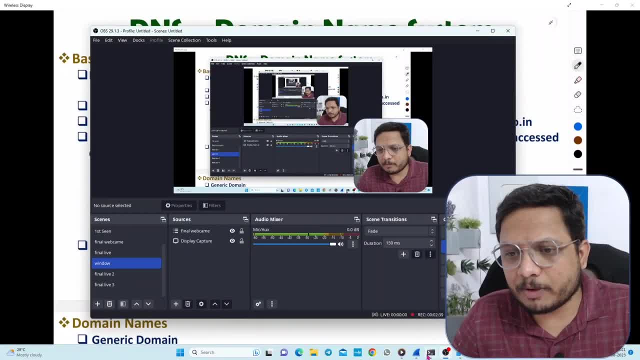 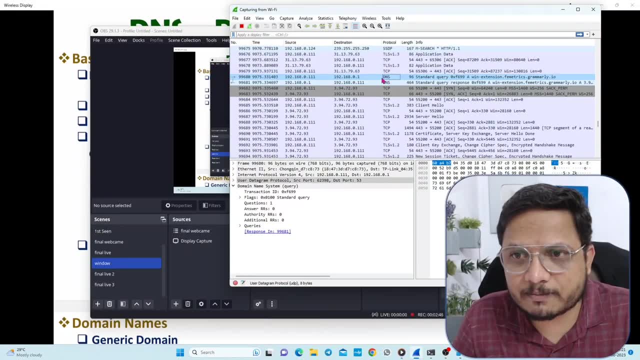 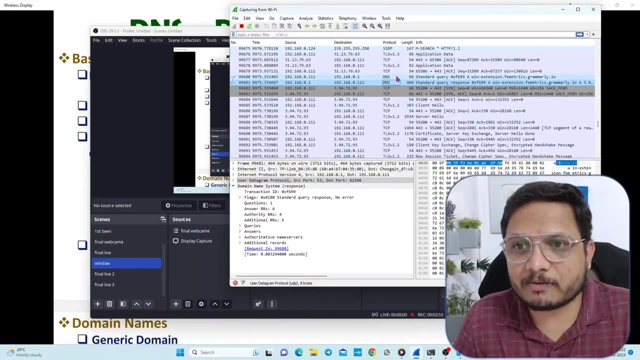 one practical scenario, so that will use you more clarity. so let me take you to my computer screen here. on my computer screen, you see, here I'll be showing you DNS protocol free. you see, this is first one and this is second one. first one is request and second one is reply. right, first one is request, you can say query. 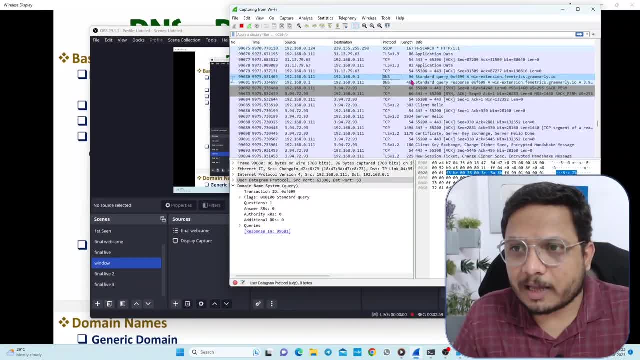 and second one is reply. now see what i was been doing. i was trying to search something on grammarly. now i i was not having, i was not having ip of grammarly, right. so you see, to access grammarly i just need to have ip to get ip i am forwarding query. so this is my ip and this is ip of my router. 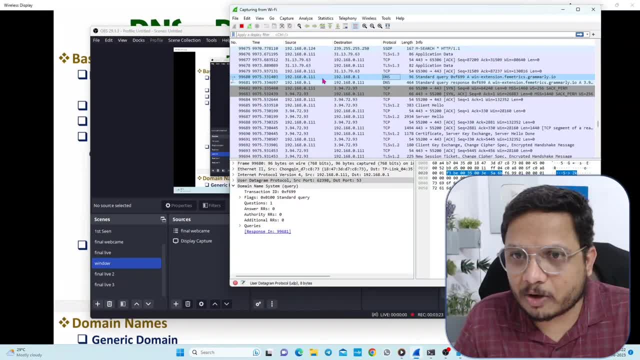 right, so i am sending frame to my router. obviously i can communicate with router only right. my router is communicating to the internet. now, see this: my ip is sending request to my router. regarding ip of grammarly, that is bns query. you see here domain name system query. that is written. 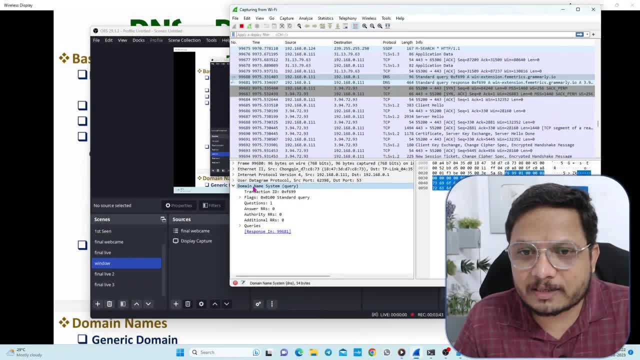 over here, right, and see this domain name system that is implemented over udp and udp is implemented here over ipv4 and that is implemented over ethernet over here, right, and then we are having frame. so this is my request. you see here query or request that you can say: that is first frame. 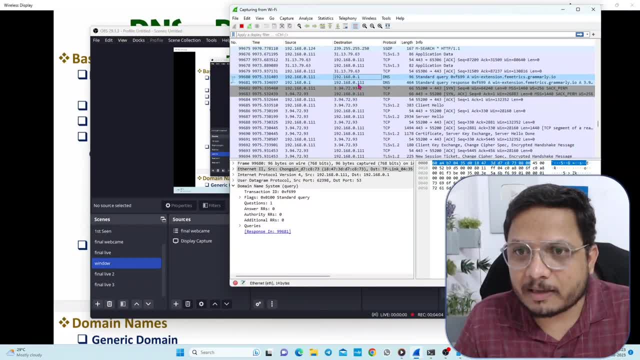 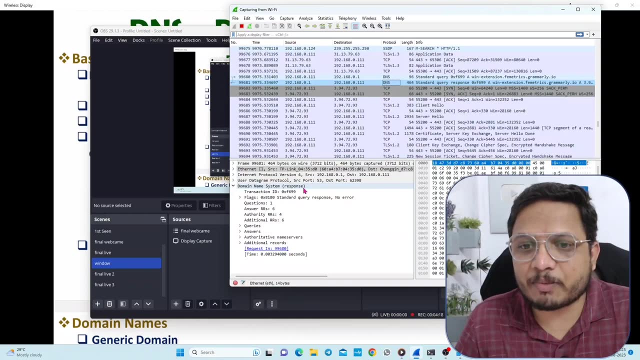 after that you see this ip, which is my ip. that is destination. ip means now my router's ip, which is source ip. now that is forwarding frame to me, that is bms, that is bms response. so by this bms response, now i am getting ip. 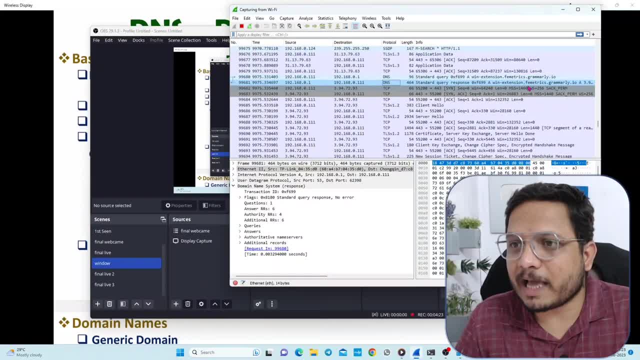 of grammarly. right now i am getting ip of grammarly. now, once i am having ip of grammarly, i can communicate with grammarly right. so see, to get ip of grammarly, i am sending frame that is dns frame that is implemented over udp protocol. remember this right. so now i think you are having idea. 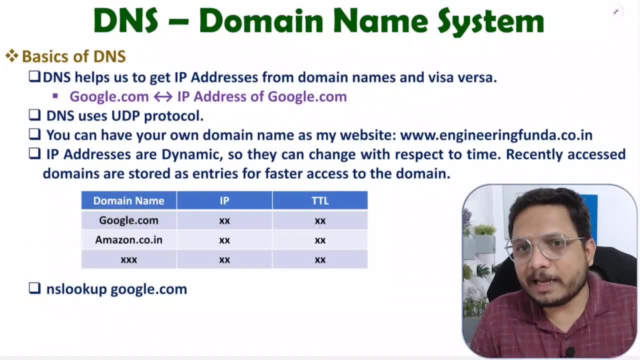 about what? what is that which we are doing right? so practically dns protocol, that we use it to get ip address from domain name right from domain name. you will be trying to get ip address right. once you have ip address, you can communicate so you can have your own domain name, as my website is there. 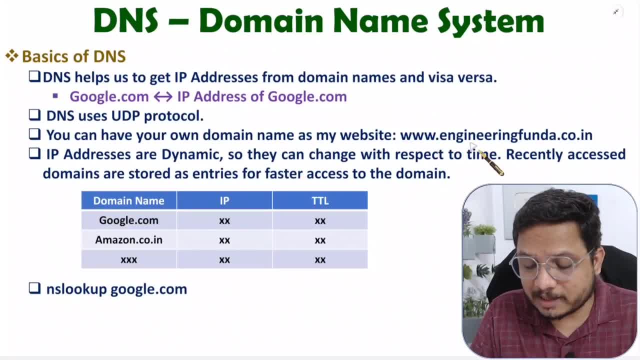 you should know that website name is wwwengineeringfundacoin, so this is my domain name right now. as if you want to access this website first, you will be forwarding dns frame along with dns protocol, so that will be request. then you will get reply. in that reply you will be getting ip of my website. 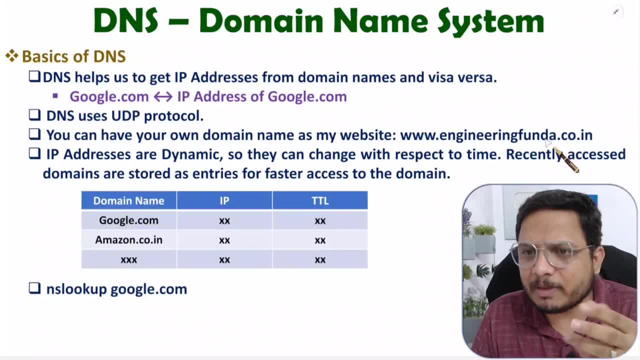 once you have ip of my website, you can communicate on my website means you can access my website right. see, ip addresses are dynamic. you should know that. dynamic means with respect to time, ip will change. before two days, when i was watching my ip of my computer, that was different compared to today. 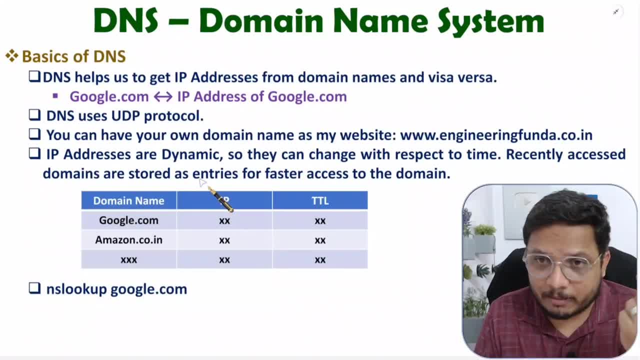 right. so ip address will change with respect to time. right. ip address will change with respect to addresses are dynamic. that will change with respect to time. recently accessed domain are stored in entries for faster access to the domain. so recently accessed domains are stored on your system right and based on that, you can. 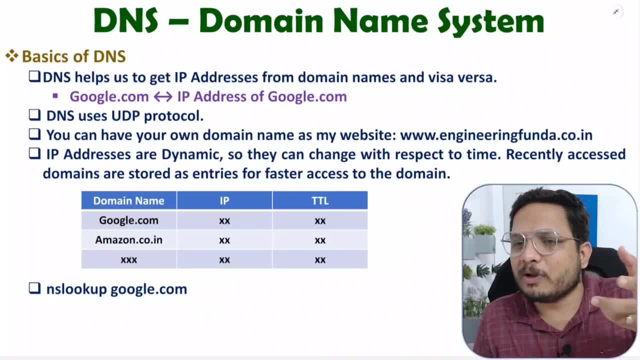 have faster access. the reason is: every time you cannot ask for domain name and all those things right do domain name that you are having, but every time you cannot ask for IP address. one time you can ask IP address. once you have it, you just store it in entries. it will not change immediately, right, it will take. 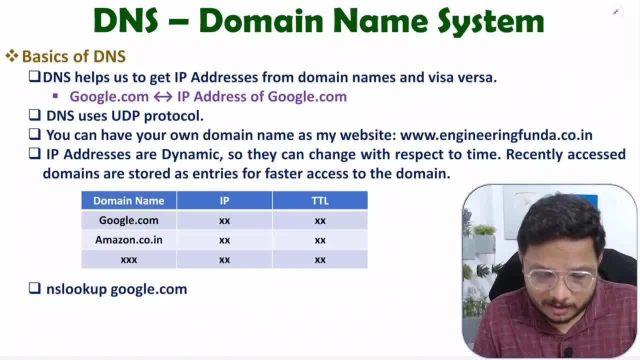 some time. so how entries are stored. let me show you that over here. see: first there will be domain name. domain name means you can have Google, Amazon or my website. that is domain name that we are storing with respect to IP address and that IP address that we get it with the use of DNS protocol and along with IP. 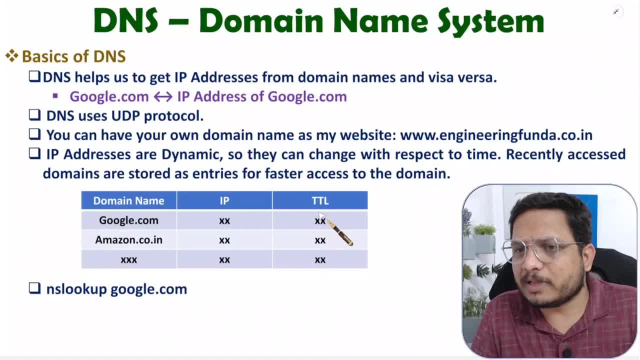 there will be validity or you can say TTL field, so that TTL field that will show you for how much time you have to wait for the domain name to be stored in your system, right? so after this time, this IP and domain name are validated with each other. after this time, both of these entries that will get invalid. 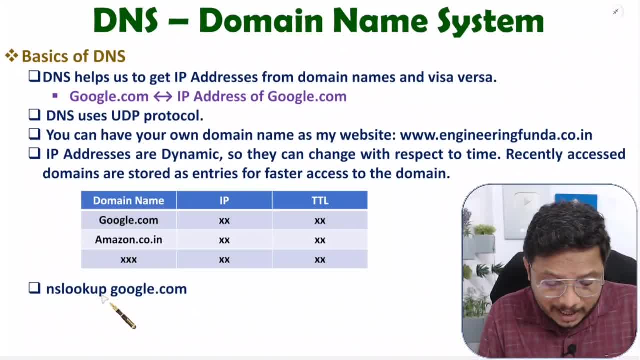 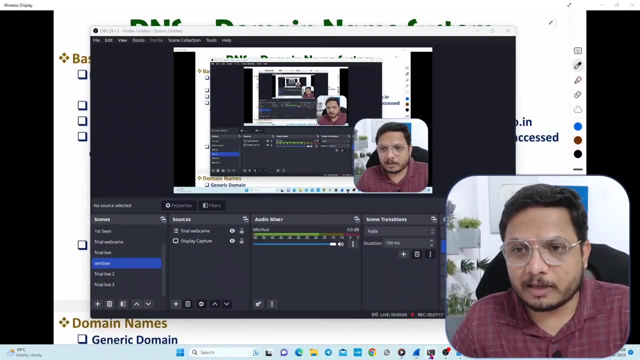 remember this right. see, one more command is there, that is NS lookup, by which you can get to know, like, how we can get IP address. and see this NS lookup that is inherently using DNS protocol, right, let me show you that on my computer screen. so here, if you observe, this is command prompt, in which I have written an NS. 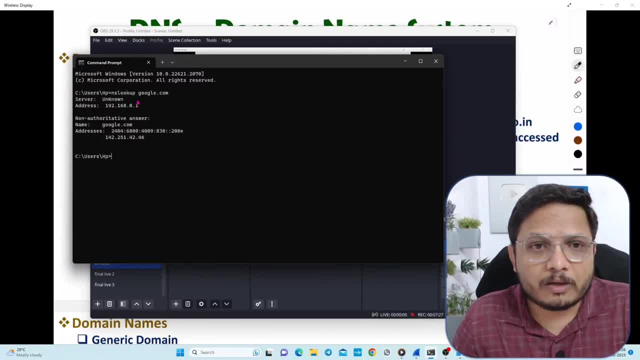 Lookup space: Googlecom. so see, this server means my Wi-Fi is my Wi-Fi is initiating that communication which is asking for IP address of Google. so you see now name: that is Googlecom. that is having IP address. that is this. this is IPv6 address languages which I have. she will need an IP address to get into Google her, not even 곰 전어い. 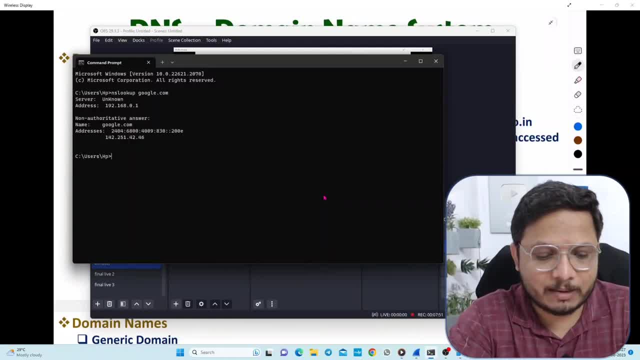 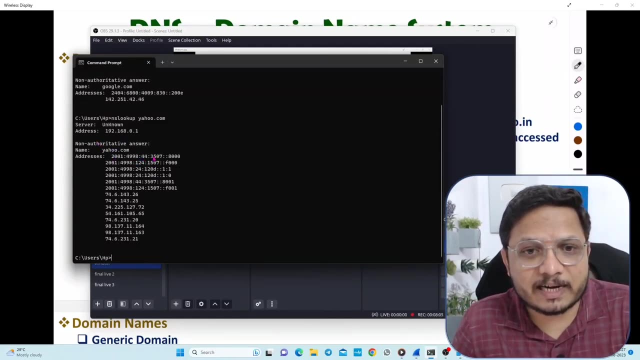 and this is ipv4 address. let me show you one more example: ns lookup space. if i write yahoocom now, you see how many, how many ips are available with this, so that many ipv6 addresses are available with yahoo. and these are ipv4 addresses are available with yahoo, with which my computer 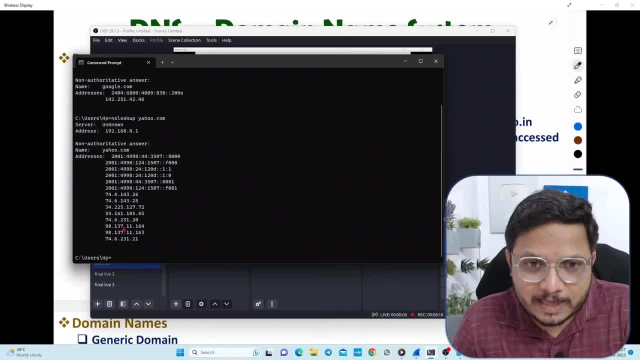 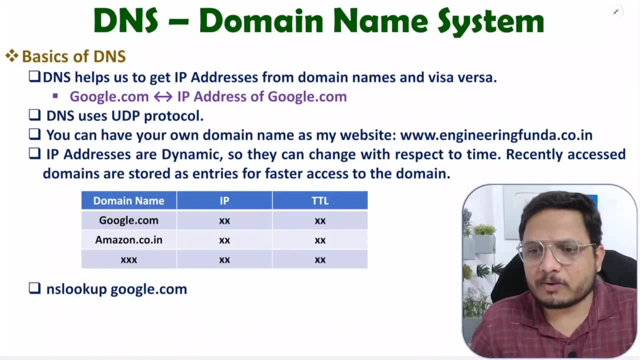 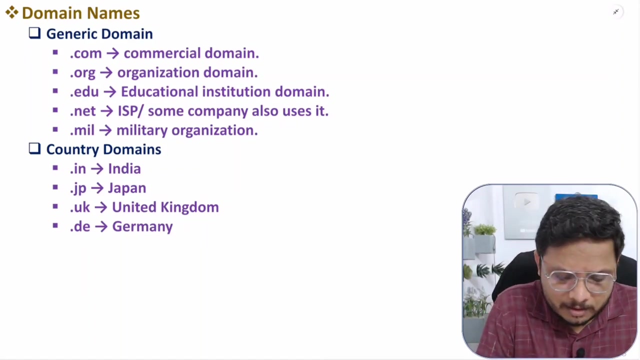 can communicate to yahoocom and to get this ip dns protocol that we are using right. so this is how things are there. so i think now you are having idea about how ns lookup is there and how dns that is working. right now let me give bit clarity about how domain names are classified: see in general you. 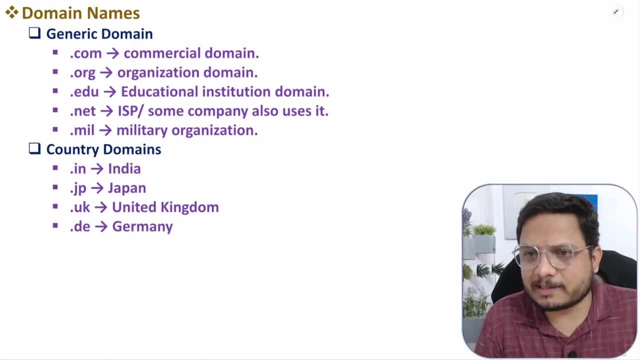 can say generic domain and country domain. that is how it is classified. these are the domain names that are classified. so let me show you one more example. these are main domain that you can see right. generic means dot com, dot org, dot edu, dot nat, dot mil. that is how generic domains are there. dot com, that is used for commercial domains. dot org is 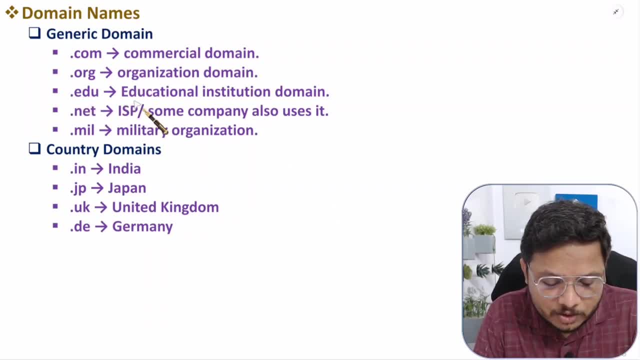 used for organizations. dot edu: that is used for educational institutions. dot nat: initially that was used for internet service provider only, but nowadays some companies are even using this. dot mil that is used for military organizations- nowadays, probably with rare use. that is there right country domains? are there country domains? 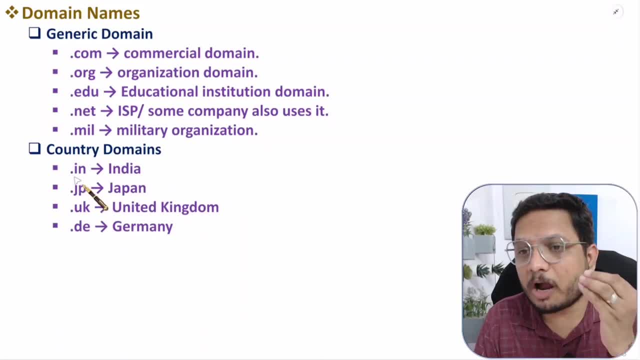 like with indiain is there, like my website, dot co, dot in. so last, at last, dot in is there that belongs to country india at last. if dot jp is there that belongs to japan at last. if dot uk is there that belongs to united kingdom at last. if dot de is there that belongs to germany, right. so that is how. 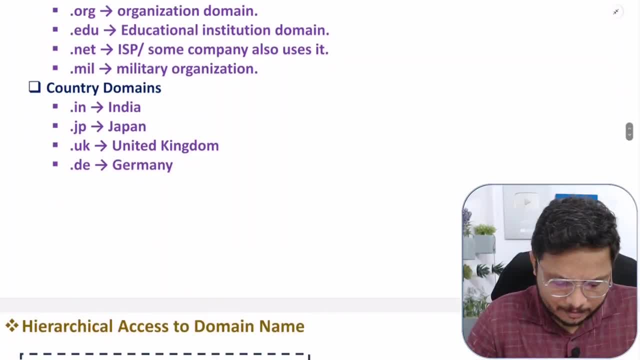 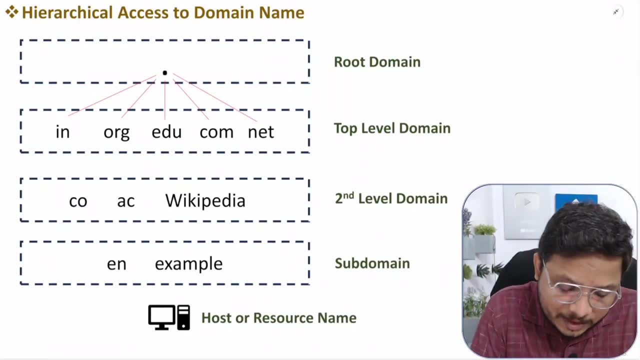 country domains are. their generic domains are there right now. let me explain you how hierarchical axis that is there with domain. so first thing that you need to understand that is this dot: this dot explains root domain. this dot that explains root domain. then top level domain will be there. at second level means after root domain there will be top level domain, totally top level. 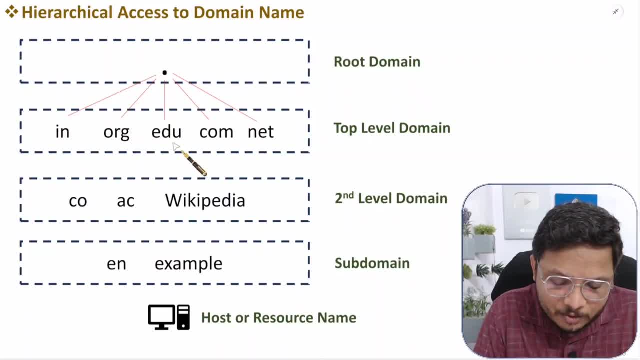 domains are like dot in, dot orged, dot com, dot, net, dot, uk, right, so those are top level domains. right after that there will be second level domains. second level domains are like dot co, dot, ac. you might have seen that even right like my website, that is dot co, dot in, there can be dot ac, dot in. so these are second level. 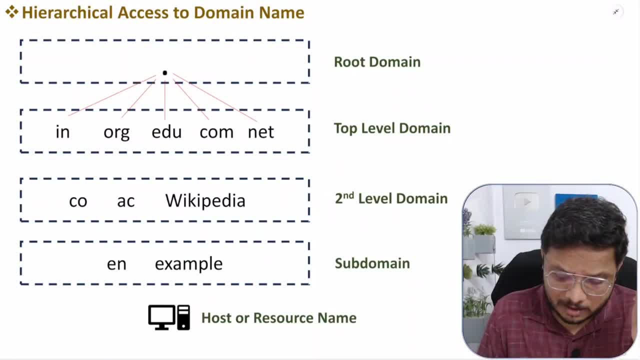 domain- wikipedia is also second level domain- and then there will be sub domain. sub domain could be like en example. let me show you one practical example, so that will give you more clarity, right, like you see, if i write engineering funda, if i write engineering funda. 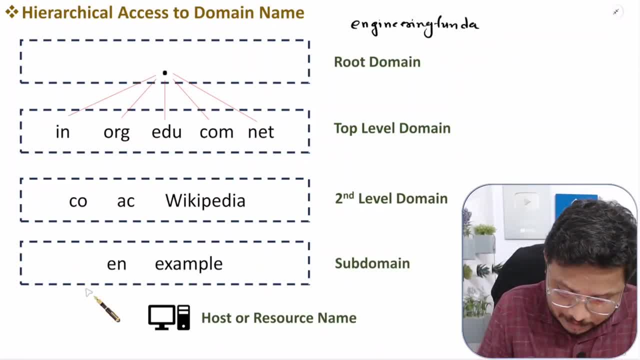 so that is my, that that is my sub domain. the reason is i i am taking it from godaddy, right? so godaddy have provided this sub domain to me. and then there is dot co, so dot co, that is second level domain. and then there is dot in right. 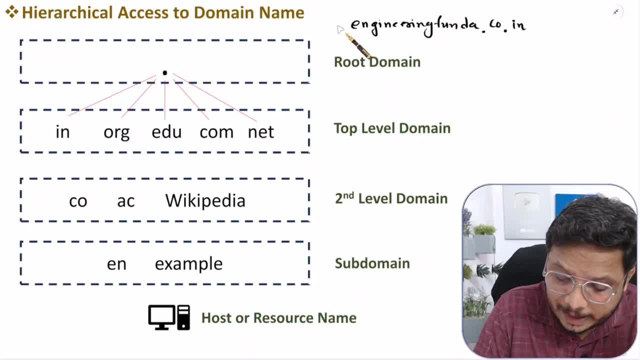 so see, this is my in total domain name where this dot, this first dot, that is domain root, then dot in is there, that is top level domain, then dot co is there, that is second level domain, and then sub domain that is engineering funda dot co will be the second level domain. so that is my sub domain world domain. i am taking it. 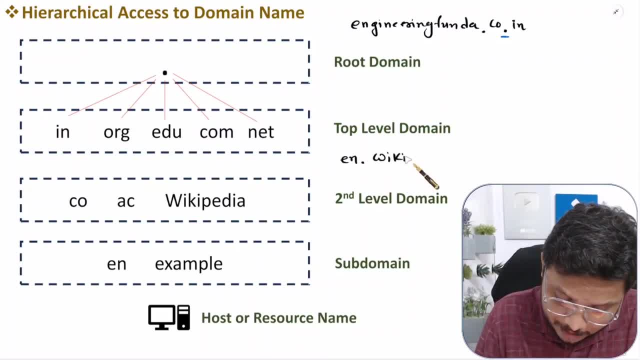 from godaddy. okay, so let me give you one another example. see in another example. what i'll be doing is i will be writing en dot, wikipedia, dot org. right, so now, if you observe here this first dot, this first dot, that is root domain, then dot org, that is top level domain, and then see wikipedia, that is. 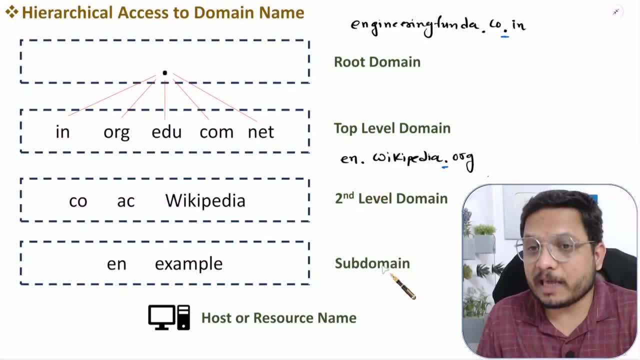 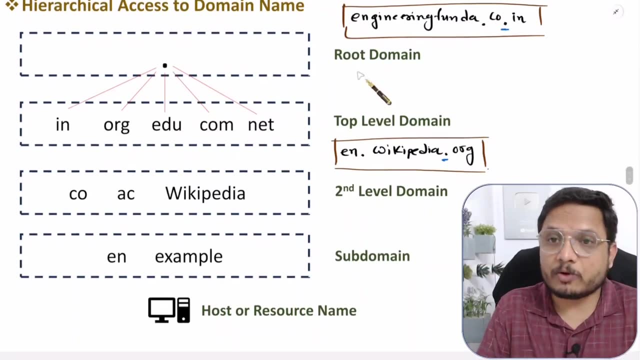 for English. so that is my sub domain with Wikipedia, and then one can communicate with host system, right? so see, this is how, this is how, two examples that I have conveyed to you. so you should know how hierarchical axis that is happening, right? so root domain is there, after that top level domain. 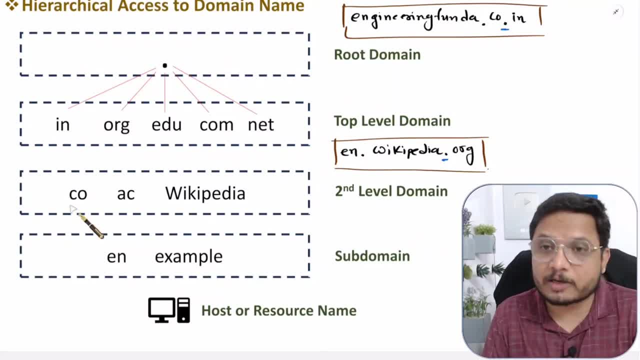 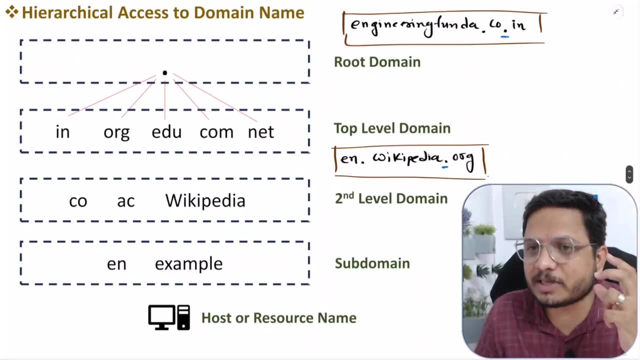 that is how this top level domains are there, then second level domain like dot, co, dot, EC. those are second level domain and then en, example. that is how some subdomains are there, right sometimes, like my website is subdomain. so sometimes what happens, you know, like in competitive examination they may give. 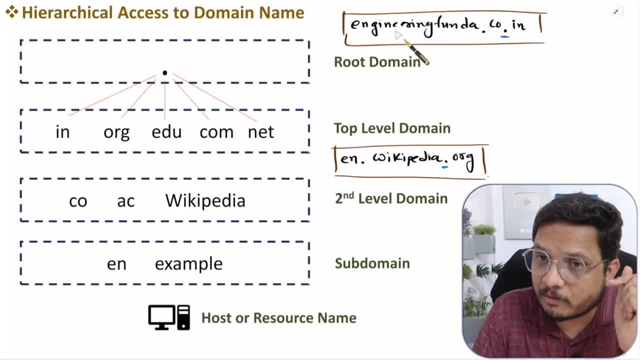 you that domain name, and in domain name there can be question like: what is subdomain with that domain name, what is second level domain with that domain name, what is top level domain with that domain name? see, that kind of questions may come in competitive example examination. so for that you should be ready, right, I think. now these two: 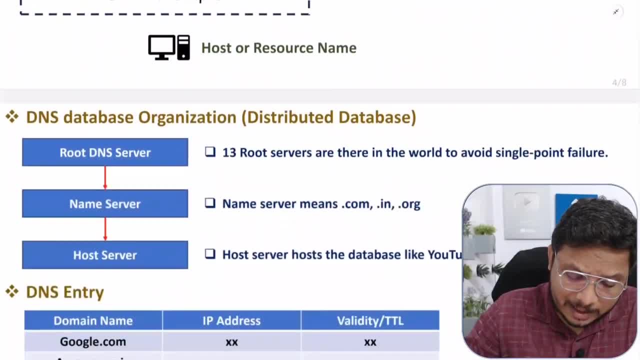 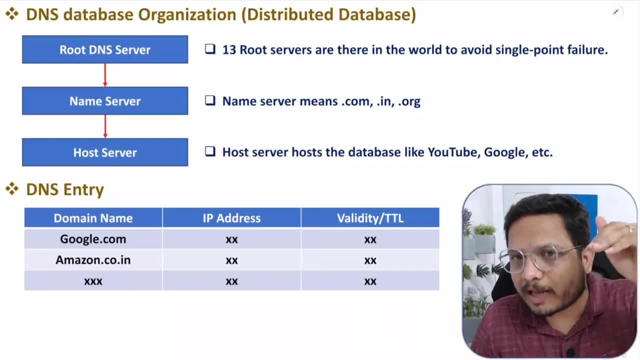 examples are sufficient to understand that. now let me explain you how DNS database organization is there. see, there are three levels of organization, that is, distributed database approach that you should write. first of all, you need to remember these three names. that is quite easy. one see root DNS server. after that. 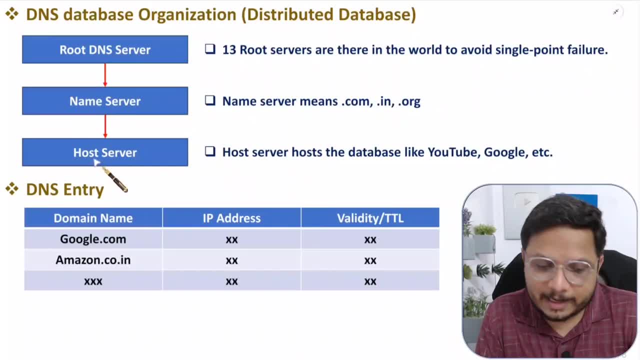 the name server and after that host server. that is how it is there: right, root DNS server, then name server and then host server. there are 13 root servers that is available in the world. and why there are 13 root servers? the reason is single point: failure is not allowed, right, like you might have seen. 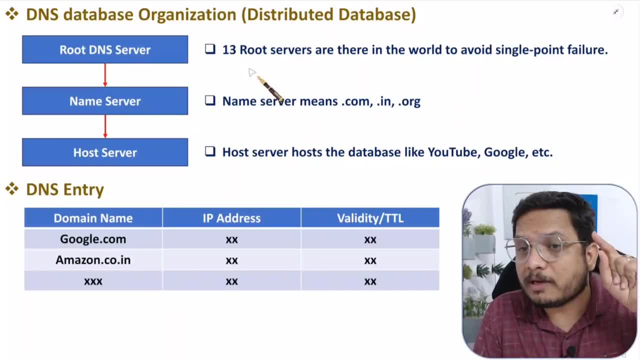 tsunami have came to Japan. now if root DNS server that is there in Japan and if single point failure is happening, then entire world's internet will go down. so to avoid those situations, right now there are 13 root level servers that is available in the globe, so single point failure will not happen. right now, root DNS server, after that there. 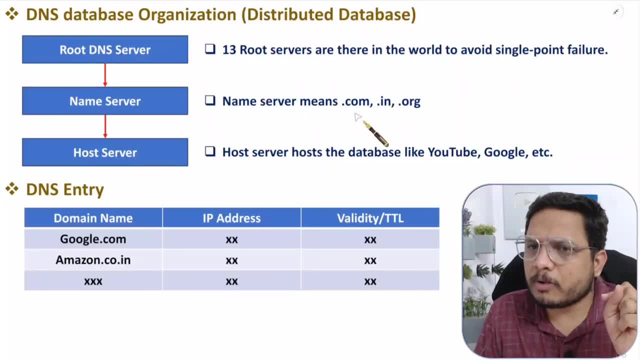 will be name server. name server is like cominorgnet, right, so those are name servers. after that, there will be host servers. host servers are like YouTube servers may be their Google server be there, yahoo server may be there. amazon server may be there, so those are host servers, right so? 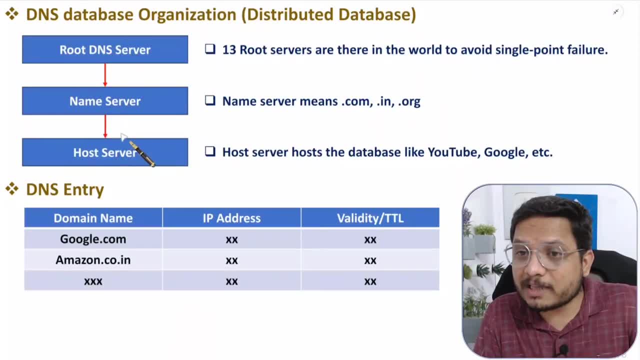 dns database organization. that is happening like this: root dns server, name server and host server. always remember this sequence. the reason is always: dns is dns. is patching ip in this hierarchy only right? i'll show you that by one practical example. but right now consider this hierarchy. 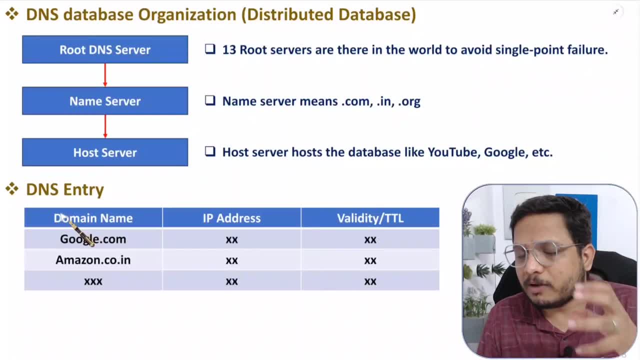 see dns entry. that i have already told you. once you take ip address from dns, there will be entry. that entry will be as per domain name, then ip address and then validity. validity means ttl. that explains you for this much duration, only this ip and this domain name. those are actively. 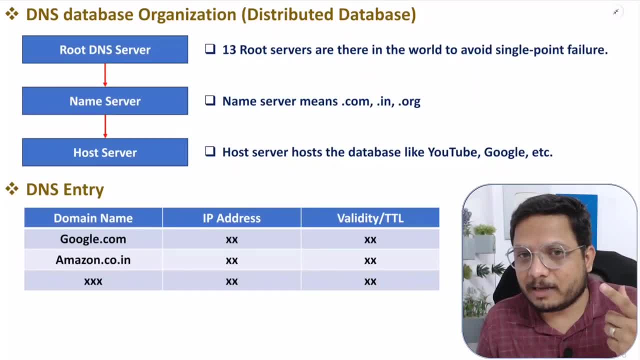 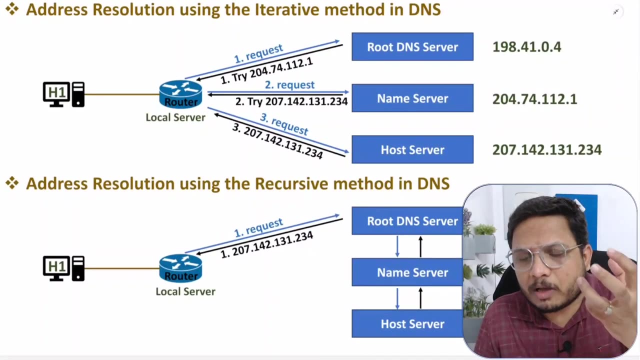 attached to each other. after that that will get invalid, right? so that is how dns entries, that is getting stored, and based on that only, we are communicating on computer network. now very interesting part that i'm going to explain you. that is address resolution means how computer is taking ip address with the use of dns. you see here one computer that i have shown. 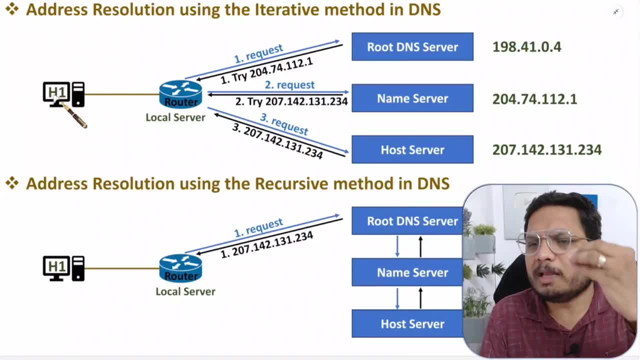 now this computer is requesting for, let us say, any website. right, so obviously, to access website with the use of dns. first, what we will be taking ip address of that website, right, but how? there are two ways. one is identity. and then we will be taking ip address of that website, right, but how? there are two ways. one is: 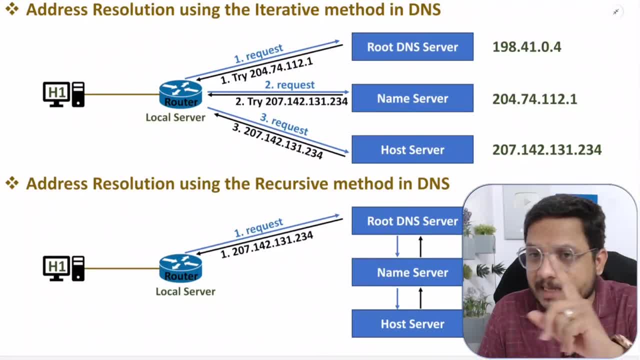 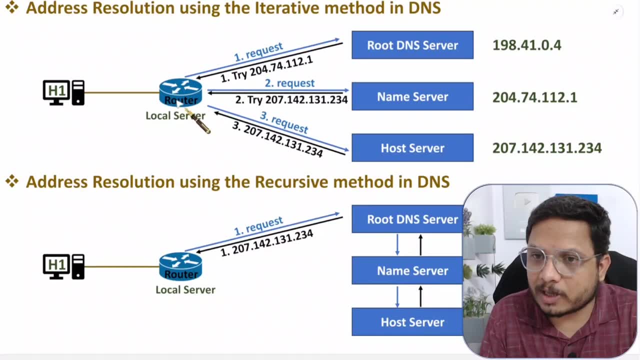 iterative and second is recursive. Let me explain you. first, iterative method. See what we do is this computer is requesting for website. that will go to this router, Like I am having my computer in front of me that is connected with my router, So obviously I can request to my router only. 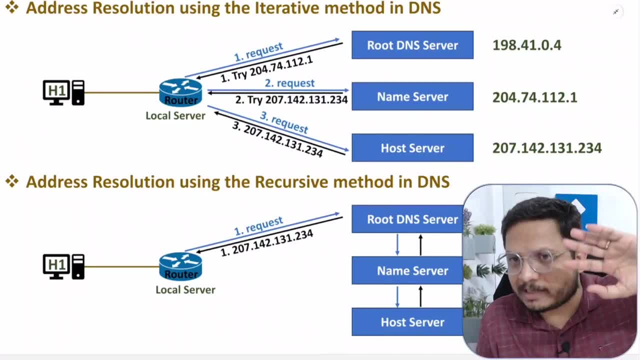 Now my router will request it to exterior environment. So this is local server, which is my router, which is connected to root DNS server. Now, you see, this router will be requesting root DNS server regarding IP. So this root DNS server is saying what Root DNS server is saying. 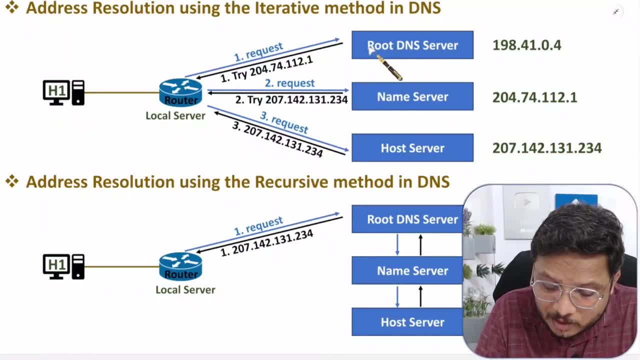 you should go to name server. How This root DNS server that will give this IP in feedback. You see this IP in feedback. So now this IP that is there with this local server, So it will send request to this name server. Now this IP that is there with this local server, So it will send. 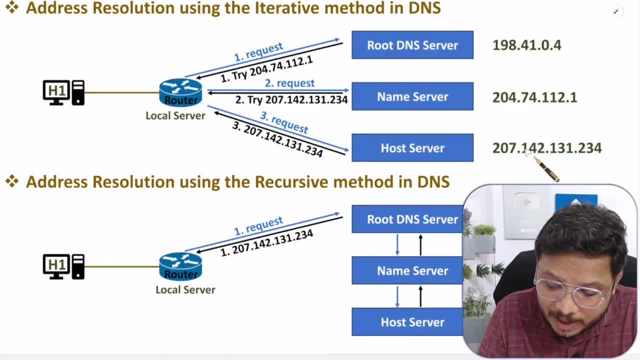 request to this name server. Now this name server will give this IP to this local router. So now this IP, now that came to this local router, Now it will request to host server. Now host server will say: OK, this is my IP. only you can communicate with me over here. 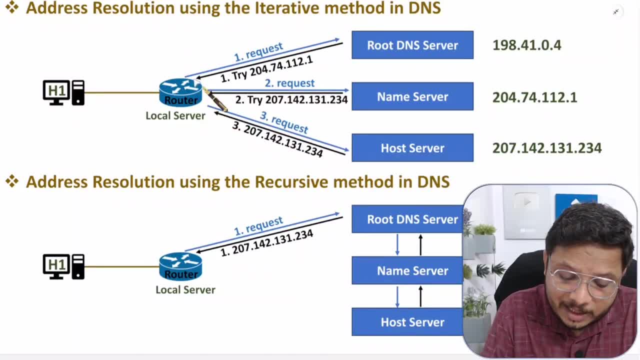 Right. So if you observe, here we are having iteration. Three iterations are there. First iteration: that have happened with root DNS server. Root DNS server have given address of name server Like See root DNS server that is having that is having database of everything, right, like root DNS server is saying you should go to dot com. 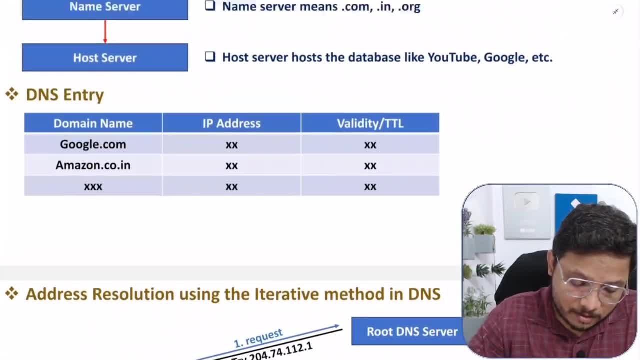 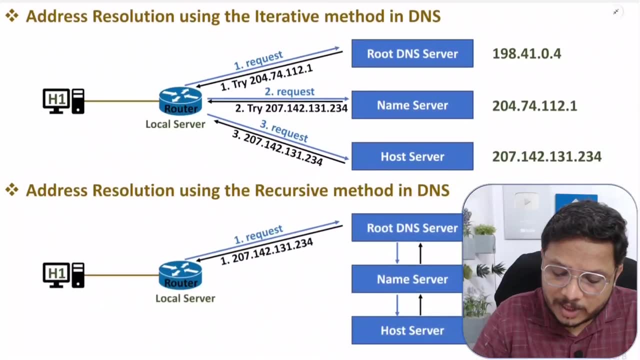 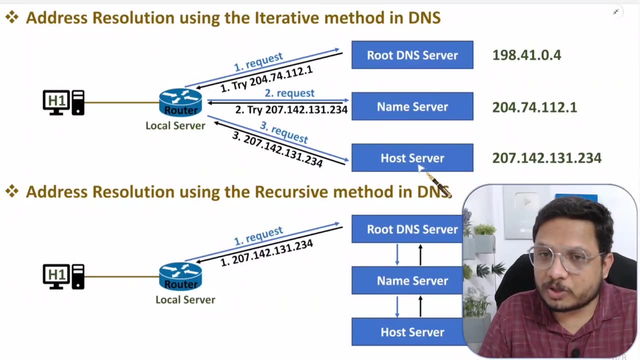 So dot com, that is there with name server. I have told you see this name server, that is, that could be dot com, dot in, dot org, dot net, right? So root DNS server. that is giving approach to name server. So name server again is giving approach to host server. 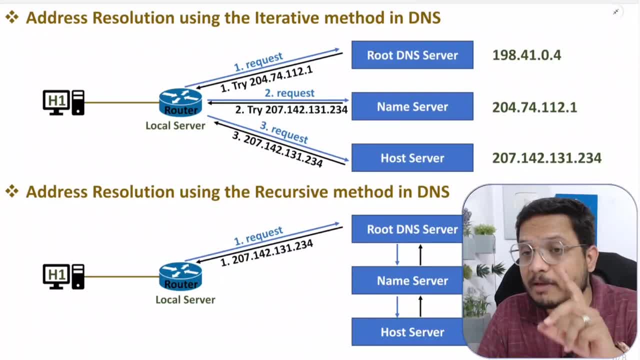 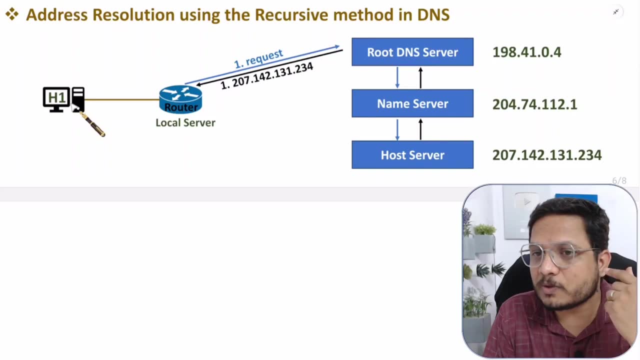 So in iterations that is happening. That is one way by which this DNS will give IP of website to host. right Now, second approach is quite interesting. You see what is happening when this host is requesting for websites IP with the use of DNS. at the time this local server is requesting this DNS server. 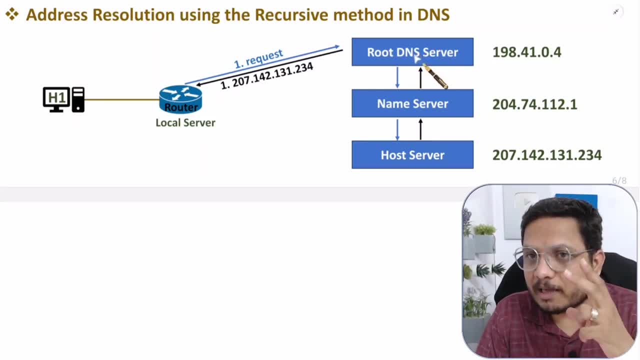 Now this DNS server is not having idea about what is the IP. So what it does is now it will not give feedback directly over here. What it does is it will ask to name server. Then name server will ask it to host server. Now host server will deliver exact IP to name server. 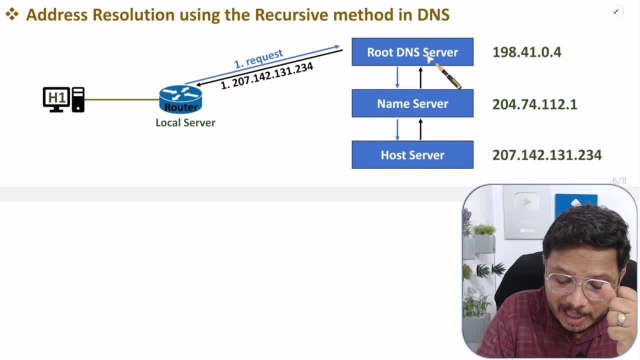 Now name server will deliver that IP to root DNS. Now that IP will come over here. So here local server is not doing iterations like this. Local server is just asking it to root DNS server. Now root DNS server is approaching in this hierarchy and it is taking that IP from host server and it is giving it to this local server. 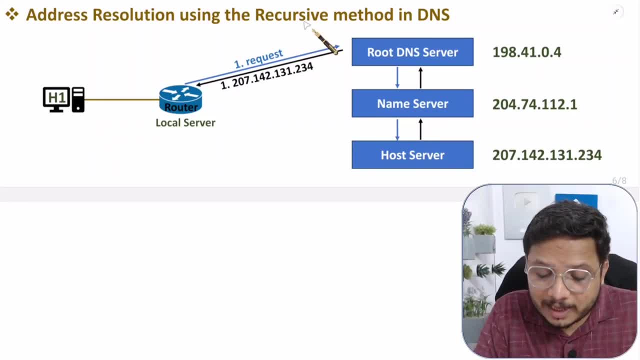 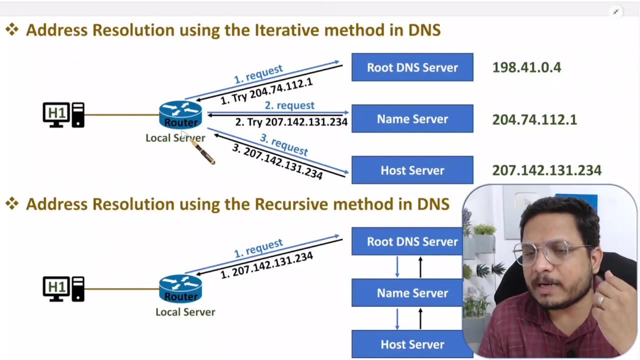 Now this local server will give it to this host right. So this is recursive method, right? So in recursive method, local server that will approach once only, while in in iterative method, local server will approach this many times. That depends on how many iterations are happening. 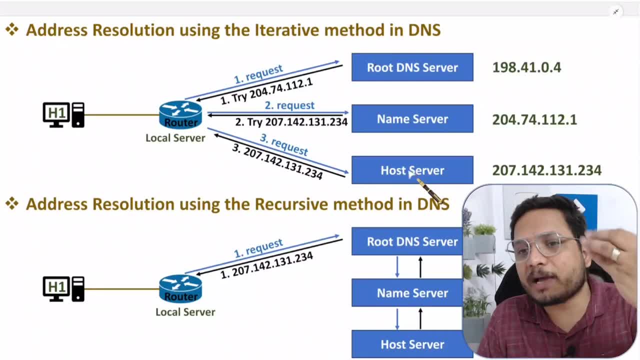 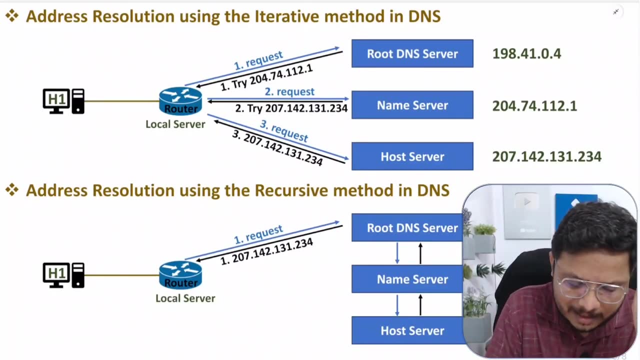 Here I have shown you three level hierarchy. right, There can be five level hierarchy. Obviously, that is always possible, right? So that is that that is possible over here in iterative. So this is how address resolution that is happening. in short, you just need to understand one thing, as if this computer is writing googlecom, then this is domain. 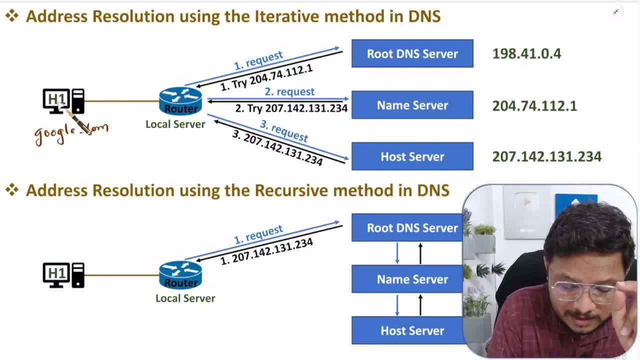 Now this computer wants IP, So this request will be given to local server. Now it will request like this, or it may request like this: right, That depends on the approach. There can be iterative method or there can be recursive method. right At last. 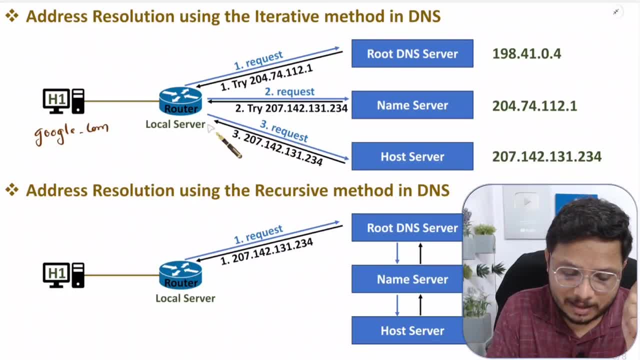 This computer will get what. it will get this IP right at last. But how much time, how long it will take, that depends on which method that we use. in iterative method, it will take bit more time. in the recursive method, it will take bit less time. 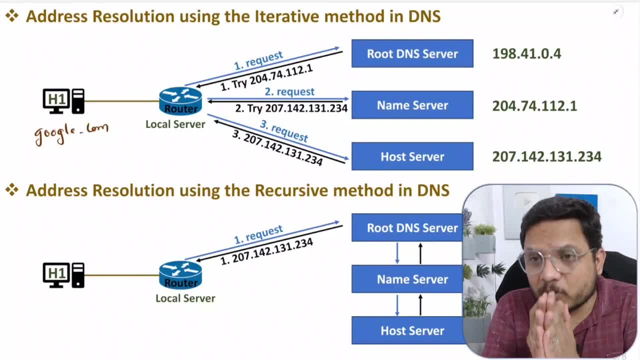 That is how things are there. If anything that would like to share, please note it down in the comment section. I'll be happy to help you. Thank you so much for watching this video. 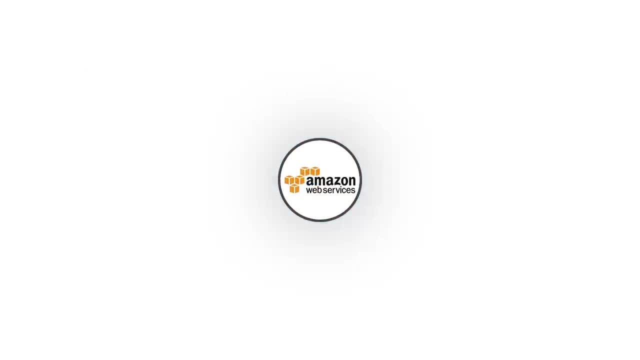 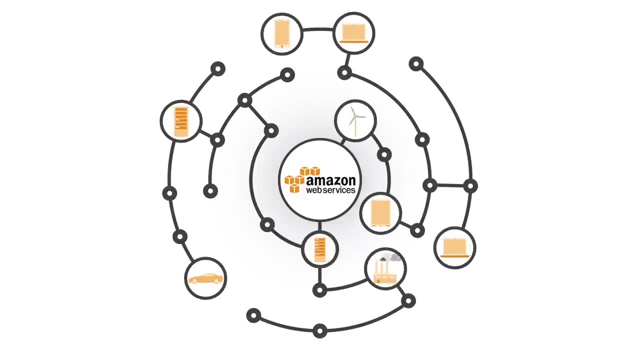 You can turn data into an innovation engine, and Amazon Web Services can get you there. Making sense of increasingly growing numbers of data sources and new devices connected to your business, customers and employees makes big data a priority for companies like yours every day. 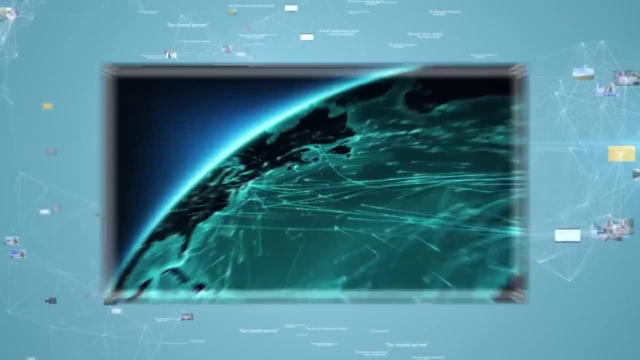 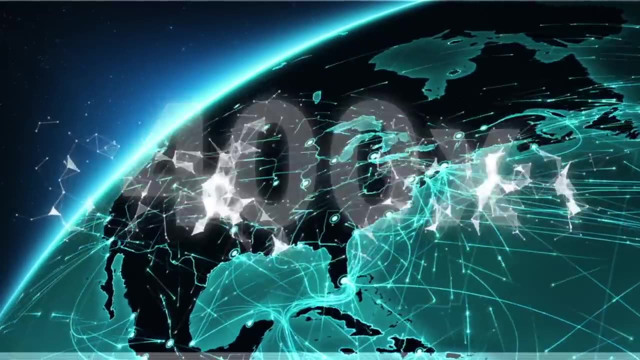 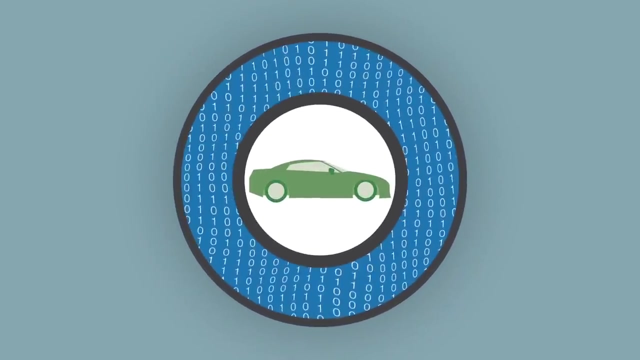 By accessing Amazon's scalable data services, companies have the velocity to stay ahead of new data demands- up to 400 times faster than on-premises solutions. all the way from a few terabytes to exabytes, With data lakes implemented on AWS- information from vastly different sources. 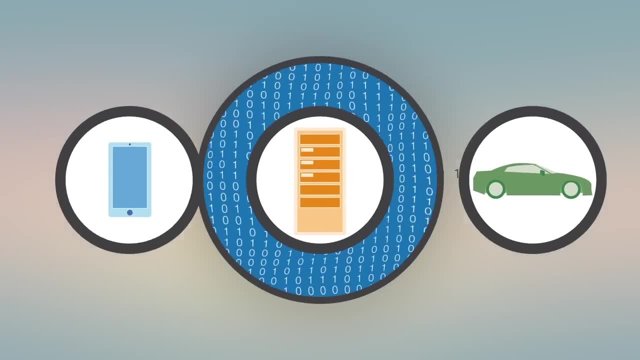 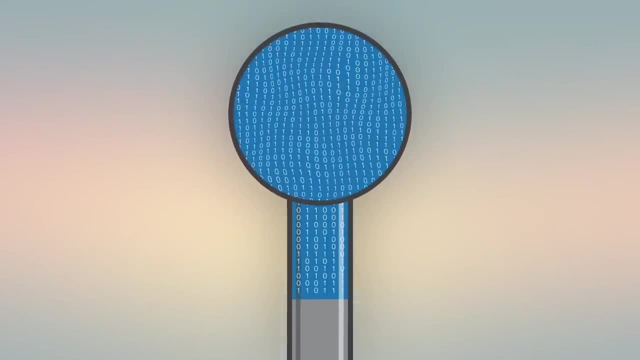 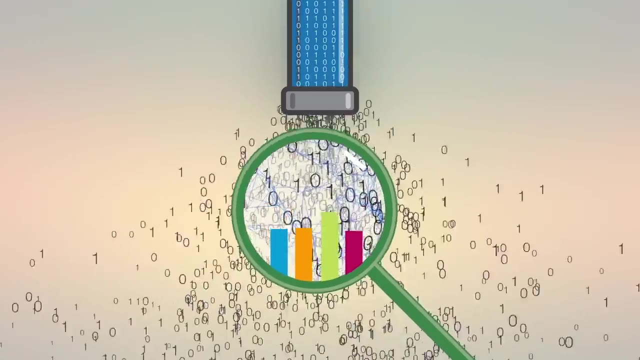 can be made readily accessible in native formats, keeping your data ready for analysis. Your data arrives continuously, millions or billions of events at a time, and you need to gain insights from this constant stream of data in real time, continuously collecting and analyzing. AWS makes it easy, with a complete set of managed services You can take.